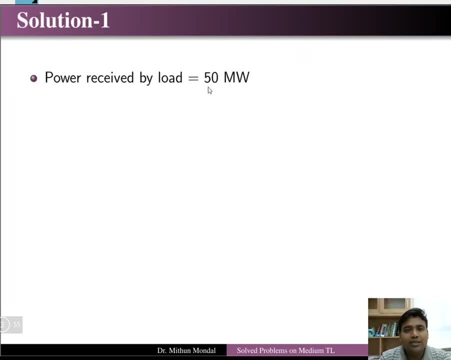 So let us see Now. the power received by the load is 50 megawatt, So what is the current at the receiving end? So if you have a load where the power is 50 megawatt, So what is the current flowing here? 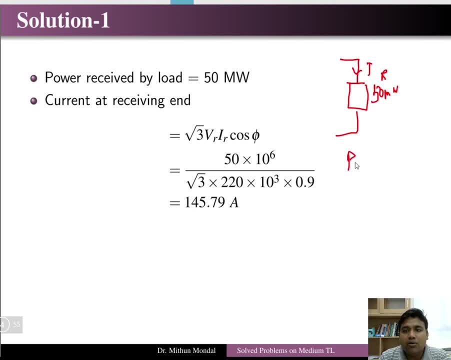 I are. Now we know that the power is basically root three times the line voltage, line current and cos phi. So here We can find out what is the value of the line current, because the power is being given as 50 megawatt, that is the three phase power, and the line voltage is already given as 220 kV. So what? 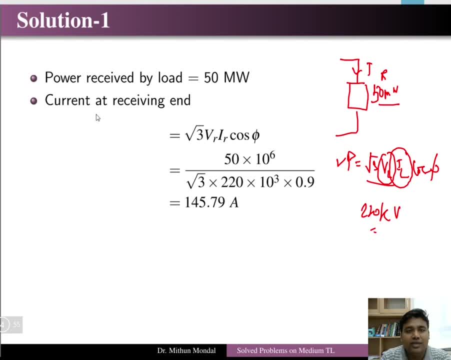 is the value of the line current, that is the receiving end current. So root 3, VRIR cos phi put the values of the power. So this is the power formula. So here from where you can find out the current, So 50 megawatt and 220 kV that we have to substitute to find out the current at the 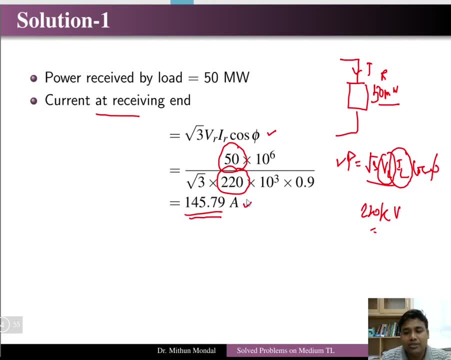 receiving end. So the current at the receiving end is 145.79 Ampere. Next, the power factor is given to be 0.9.. It means the phi value, that is, the angle between voltage and current, is 25.9 and 25.84.. So the receiving end current in terms of the vector is 145.79 Ampere, which we have. 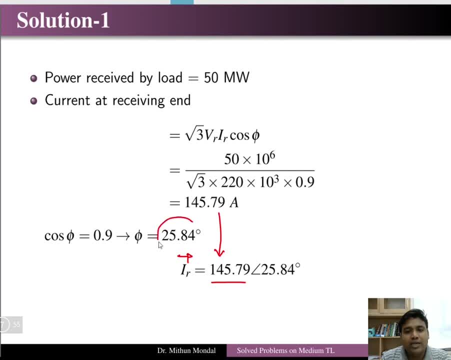 calculated is the magnitude and 25.84 is the angle, because we have taken the reference is to be the VR. So VR is taken as the reference, which is at zero degree. So here it will be at 25.84.. Now the value of VS. 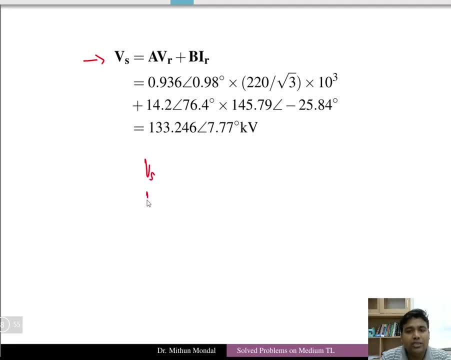 we can calculate it from the abcd parameter. we know that the sending and voltage- sending and current- is related with the receiving and voltage and receiving and current with the abcd parameter. so the sending and voltage we can get as avr plus vir, where the parameters a and b are already given. 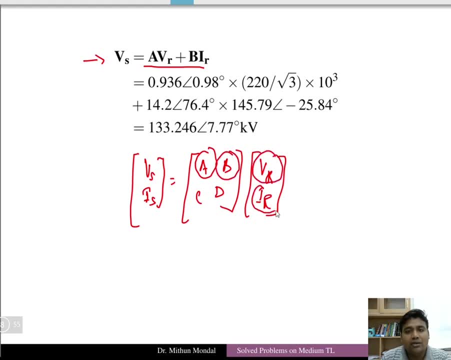 and vr is given to you and ir we have calculated. so this is the value of the sending and voltage. then this value is corresponding to single phase. this value is corresponding to single phase because all calculations we are doing in single phase. however, the question is asked: what is line? 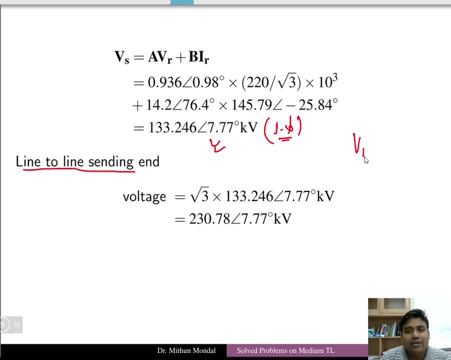 to length sending end. so we know that the line voltage is equal to root three times the phase voltage. so multiplied the root three with the magnitude of 133.246, the angle will remain the same. so you will get an answer of 230.78 as the magnitude of the three phase line voltage with. 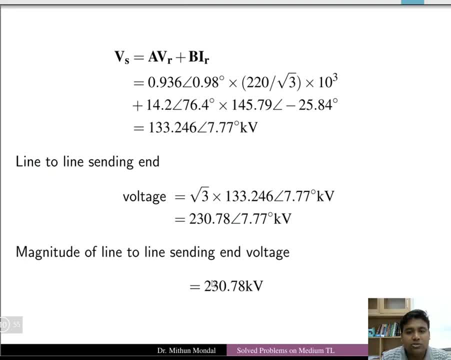 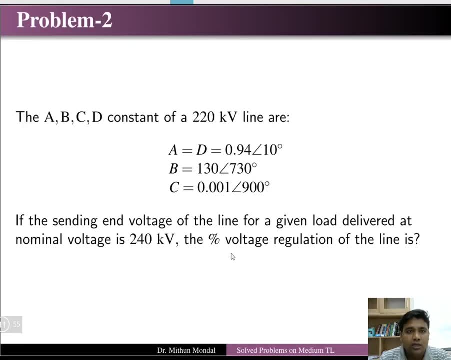 an angle of 7.77, so the magnitude is 230.78 and that is your answer for the sending and voltage. the next problem that we are going to solve is, given the abcd parameter of a 220 kv line, if the sending and voltage of the line for a given load delivered and the 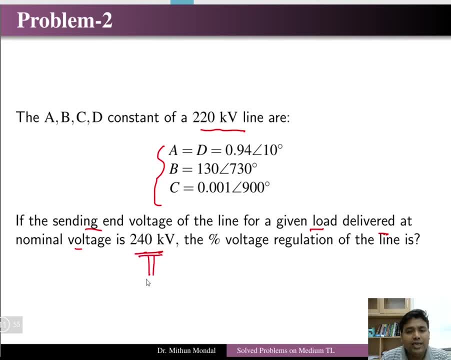 nominal voltage is 240 kv. so 240 kv means it is the sending and voltage, the percentage voltage regulation of the line. so you have to find what is the percentage voltage regulation of the line if the abcd parameters are given and the sending and voltage is given. so the voltage regulation of 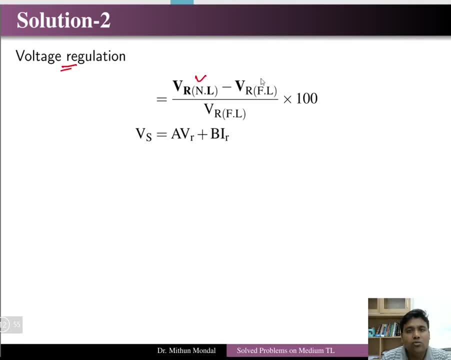 the line is given by the percentage voltage regulation of the line. so the percentage voltage regulation of the line is given by the formula voltage at no load minus voltage at full load, by voltage at full load into 100, whereas we take the reference as the receiving end, so corresponding. 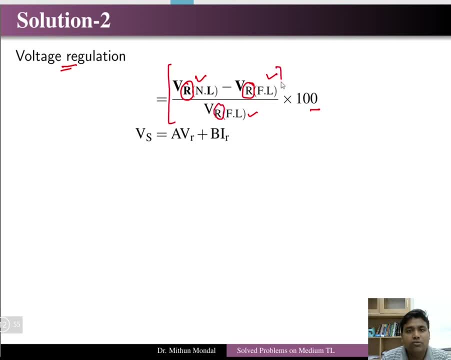 to the receiving end. we are trying to find out the voltage from no load to full load condition and we know that the sending and voltage is basically a times receiving and voltage plus b time receiving and current and for no load condition your receiving and current is zero. 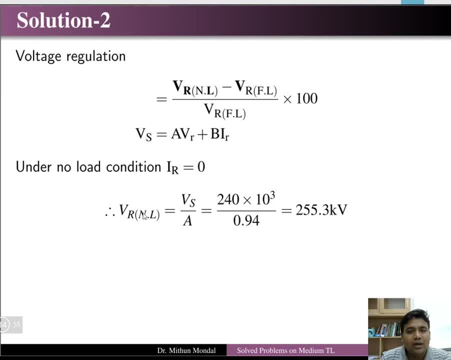 so receiving and current will be zero. then the- because here we have to find the no load condition, so no load condition- your receiving and current will be zero. then the voltage at the no load condition at the receiving end would be equal to, because this will become equal to zero. so vs by a, we have been given the value of the sending. 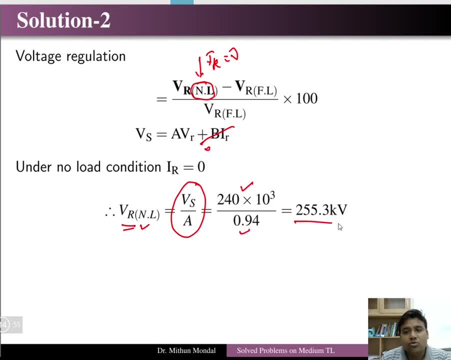 and voltage. we have been given the value of the parameter a, so we can easily find out what is the voltage at the no load condition. percentage voltage regulation of the line is given by the voltage regulation. then we can calculate as the voltage of the no load. that is we have to put it. 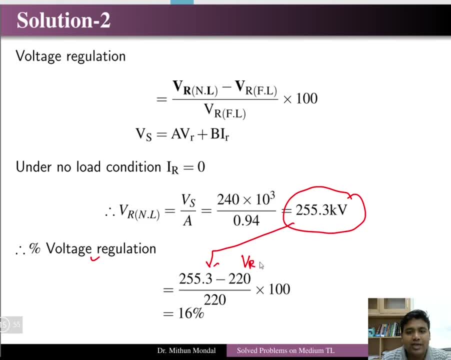 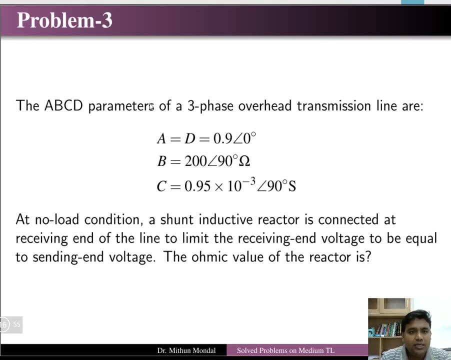 here and minus voltage of the receiving end and full load condition that is given in the question, divided by the reference as full load voltage into 100, so 16 percent, we are getting the voltage regulation of the line. so this is problem number two. problem number three: here we have been given 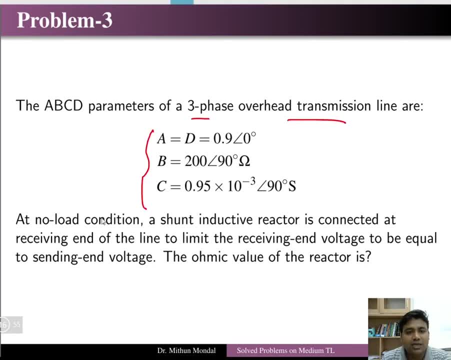 the abcd parameter of a three-phase overhead transmission line and we have been given the value of the receiving end voltage. it is given by the characteristics of the receiving end voltage as given. so at no load condition, one condition means the receiving end current to be zero. some. 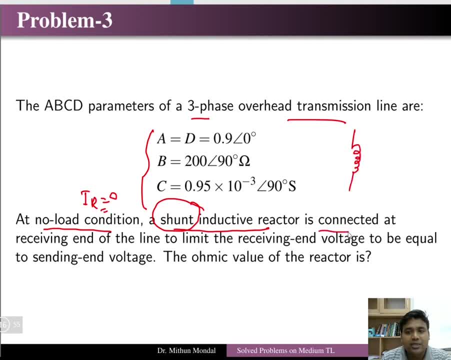 inductive reactor. something is parallel. so a some inductive reactor means you have to connect a reactor in the line is connected at the receiving end. so at the receiving end you will connect every actor to limit the receiving and voltage to be equal to the sending environment. so the condition: 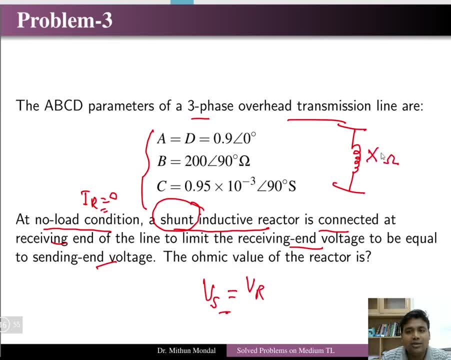 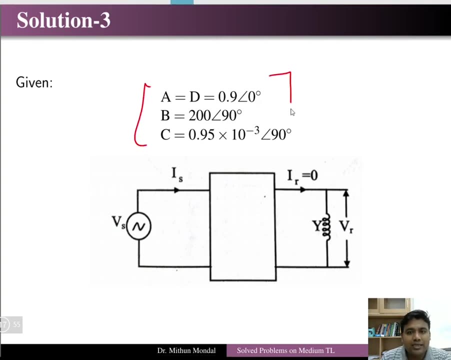 is given as ohmic value of this reactor. so what is the value of x of the reactor that we have to consider? so the case given is sending and voltage is equal to receiving and voltage. now, since the abcd parameters are given and it has been given, the sending and voltage is receiving and voltage. 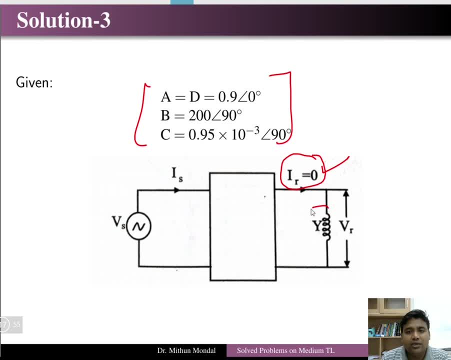 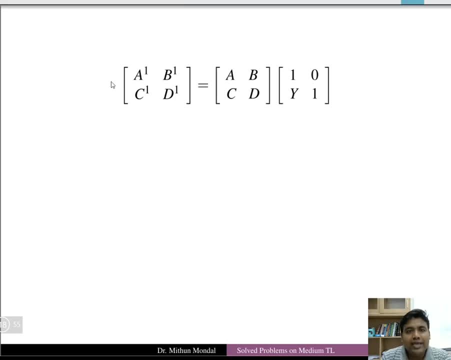 under no load condition. your receiving and current is zero, and here you have been connected a reactor. so at the receiving end the reactor is connected. so the new abcd parameter- so this is your new abcd parameter- is equal to the old abcd parameter without the reactor, multiplied with a reactor. 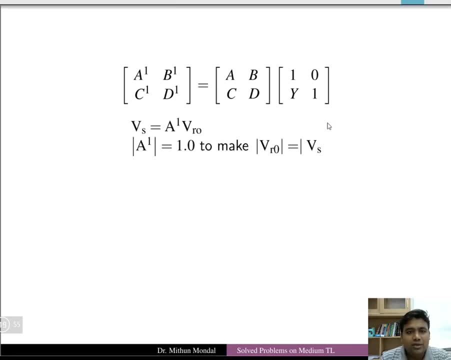 abcd. okay, so, having known that the voltage at the sending end will be equal to the new a parameter that we are going to obtain from here, multiplied with the voltage at the receiving end, under open condition, so the value of a will be equal to one, because 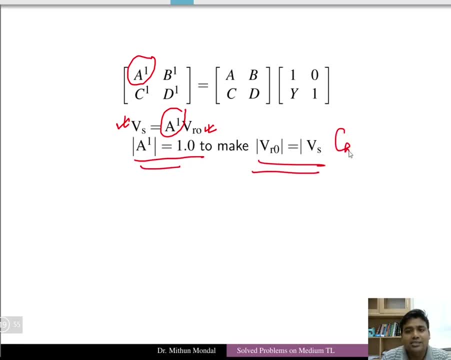 the sending and receiving end current is equal. this is the case that we have been given, so your sending and receiving end current is equal. it means your this parameter, new parameter, a, would be equal to one. so if a is equal to one, then a plus by will be equal to one, because this: 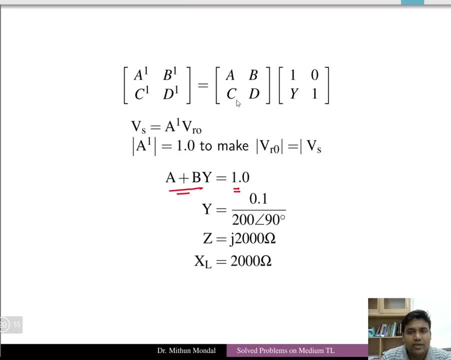 is equal to your voltage. okay, so here you have been given. if you split this, a multiplied with one plus b multiplied with y, so a plus by, is equal to a one, so a one you are having given the value of one. and why, uh, you have to find out. and then so y is basically uh, a divided by a 0.1. that is the value of the parameter a. 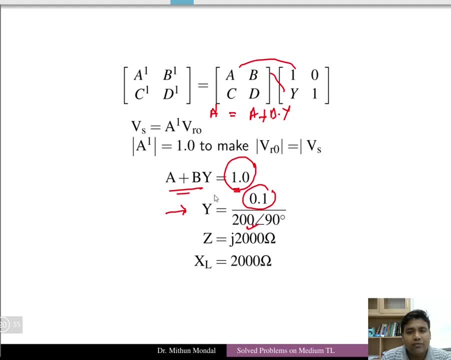 divided by the parameter of b. so after finding the value of y, you can find out what is the impedance. so impedance is equal to 1, by admittance. so you have find out the impedance and then the value of xl will be equal to 2000 ohms. 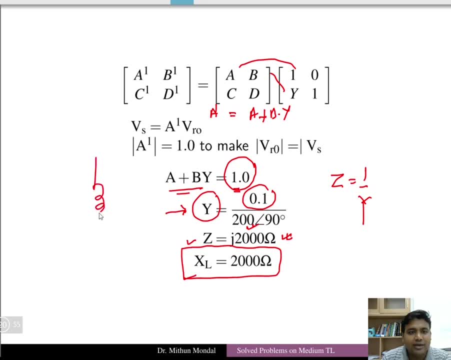 because r is 0, so the reactor that you are connecting at the receiving end- so it is xl value- is equal to 2000 ohms. so in this way we can find out, because if you have an old system and you have been connected with a new system, then your parameters together will become a new. 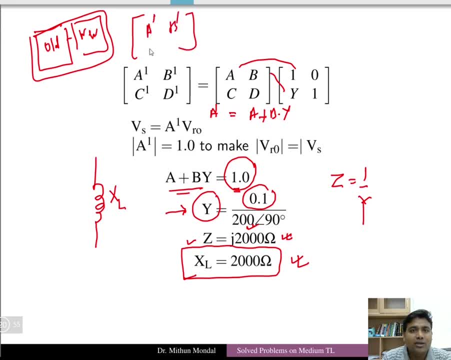 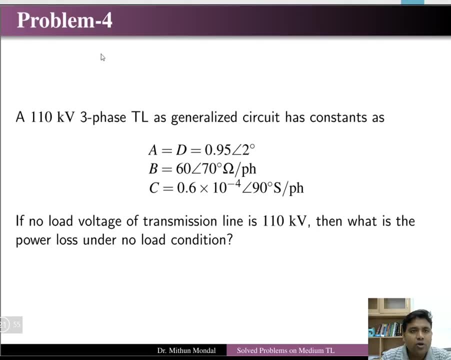 abcd parameter. so new abcd parameter: you can indicate by a dash, b dash, c dash and d dash. so this way we can solve the problem. next problem, problem number four, is basically 110 kv three phase transmission line whose abcd parameters are given if no load voltage of 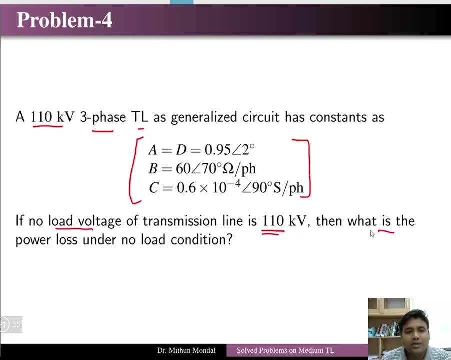 transmission line is 116, 117, 118, 110 kV. then what is the power loss under no load condition? So no load condition means your receiving end current is 0.. You have to find out the power loss under the no load condition. 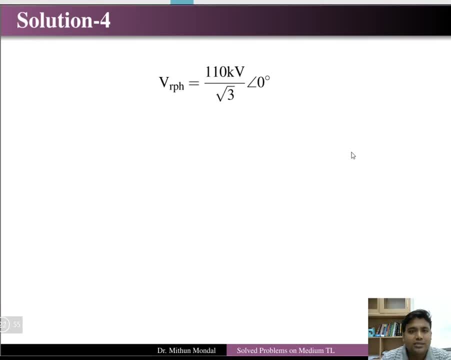 for the particular system. So let us see So the system. as you know that from three phase we will be converting to single phase. to solve it, then the voltage at the receiving end was given to be 110 kV. we have to divide it with root 3, angle is 0 because we have taken the 0. 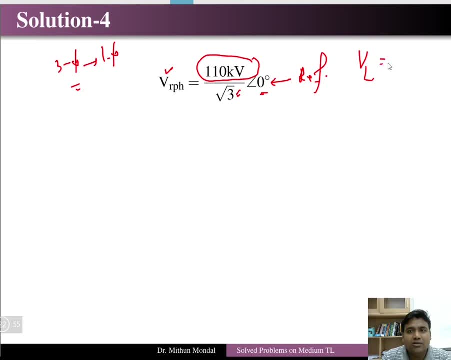 as the reference and line voltage is equal to root 3 times the phase voltage, So phase voltage would be equal to 1 by root 3 times the line voltage. Then, since the receiving end current is 0, the sending end phase voltage would be equal to A times the receiving end phase voltage. 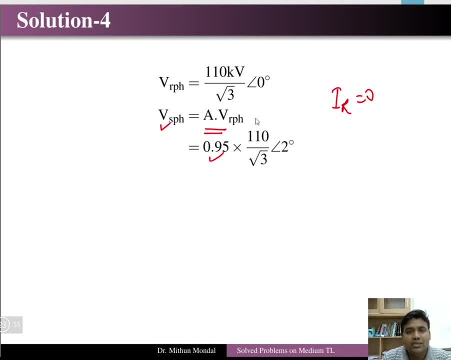 So the parameter A is given and A, So we can find out the value of the sending end voltage phase, and the sending end current will be equal to C into B V of R phase. So we can get it. So this is corresponding to. 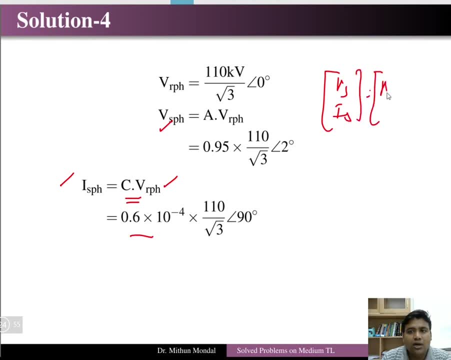 Vs Is and it is equal to the AVCD parameter of the line, whereas the Vr value will be there and Ir will be 0. So this, when splitting, we can use this equation and this equation to find the voltage of the sending end and the current at the sending, Then the 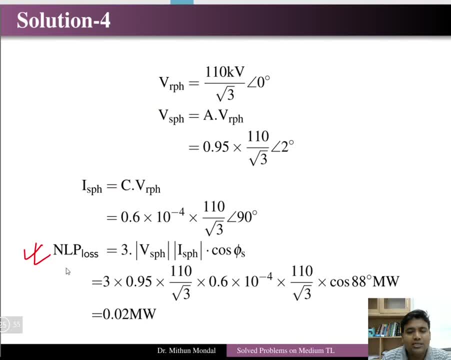 power Laws we can calculate and the no load condition as three times the sending end voltage, sending and current and the co ion of the angle between the voltage and the current. So that will give you 0.02 megawatt. So this way we can calculate the no load power. 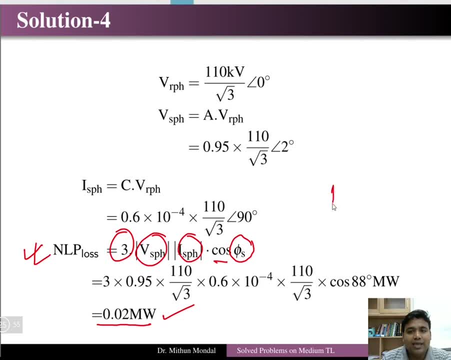 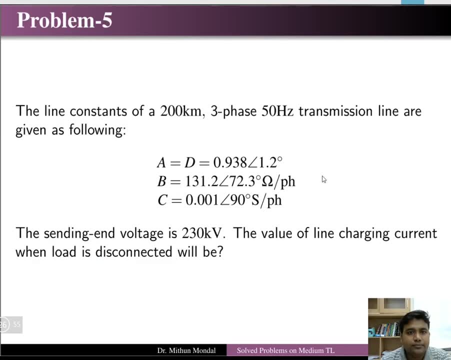 loss for a medium length transmission line When its lambda is equal to 0, if it is a, its abcd parameters are given and the conditions are that the receiving and current is zero. under the no load condition problem number five we are going to solve. so here, the line constant of a 200. 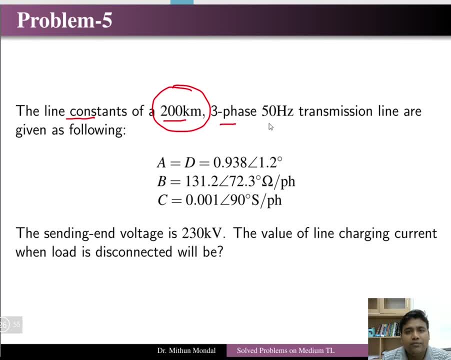 kilometer, that is a medium length transmission line of a three phase 50 hertz are given. so these are the abcd parameters, given sending and voltage is given to be 230 kv. so sending and voltage is given to be 230 kv. in the previous problem receiving and voltage was given. find the value. 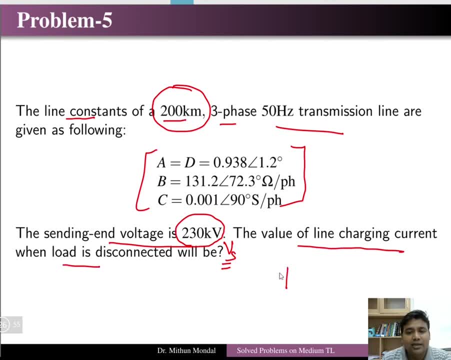 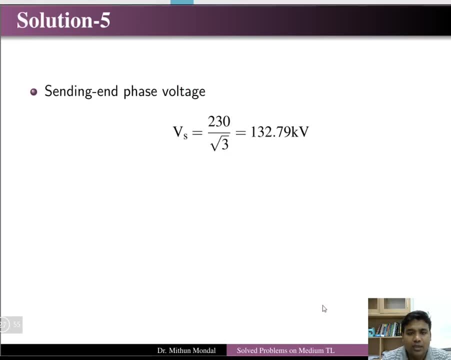 of line charging current when the load is disconnected. so load disconnected means ir to be zero. you have to find out what is the charging current of the line. so the sending and voltage. now we have to convert into per phase, that is 230 by root 3, and then the receiving and current is: 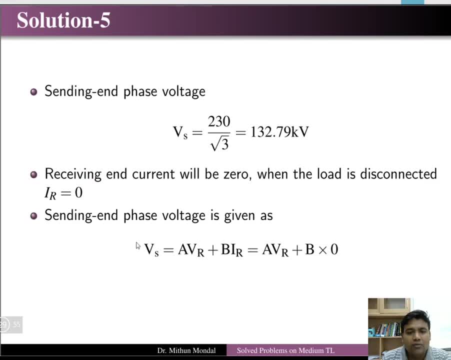 zero because the load is disconnected. so the from abcd parameters we have a relation. vs is equal to a vir plus vir where ir is equal to zero. so it means that you can easily calculate the value of vr is equal to vs by a because your ir is equal to zero. 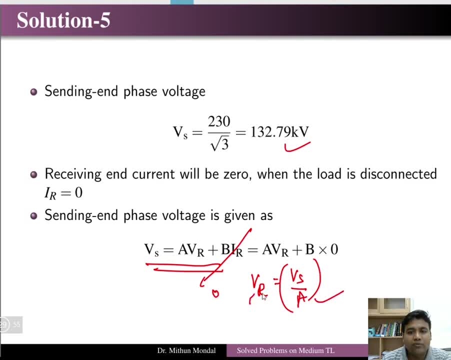 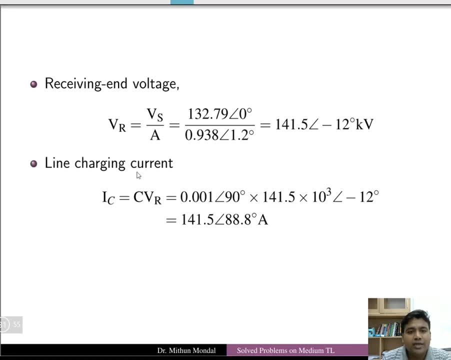 vs is already given. a is known to us, so you can find the value of vr. so vr is equal to vs by a. we can find out the value of vr. after that, we can find the charging current ic, as vr is equal to vs by a. so we can find the value of vr. so we can find the value of vr after that. 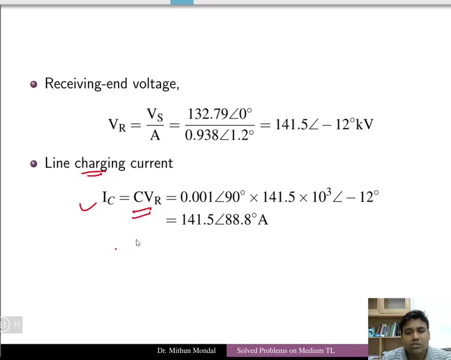 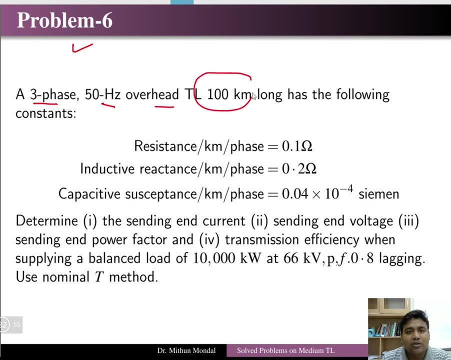 C into VR, because your IR is equal to 0. So C is known to us, VR is. we have calculated so we can find out what is the charging current of the line. Next problem, problem number 6, is a 3 phase 50 hertz overhead transmission line 100 kilometer. that is the medium length transmission line, the 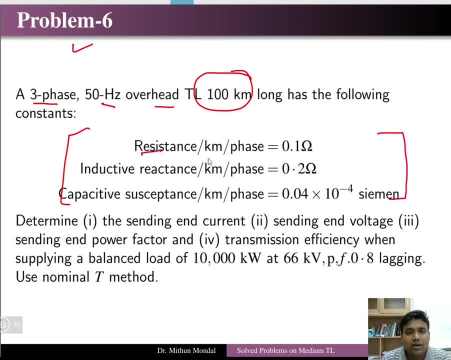 parameters are given to us: the resistance per kilometer per phase, inductive reactance per kilometer per phase, capacitive reactance per kilometer per phase determine the sending and current sending and voltage sending and power factor transmission efficiency when supplying a balanced load of 10,000 kilowatt, 66 kV power factor. So the load information that is being 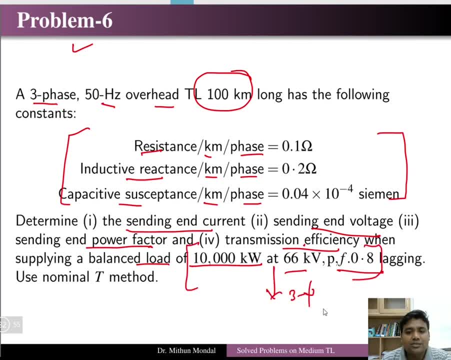 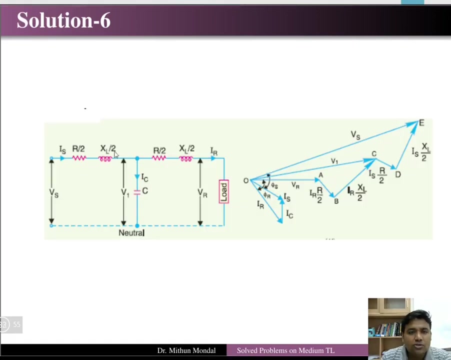 given is corresponding to a 3 phase load. you have to use the nominal T method- nominal T method to solve this problem. so the parameters are given. The difference between the previous problem and this problem is that the AVCD parameters are not given to us, rather than the parameters are given to us. So here it is the T model that we have been. 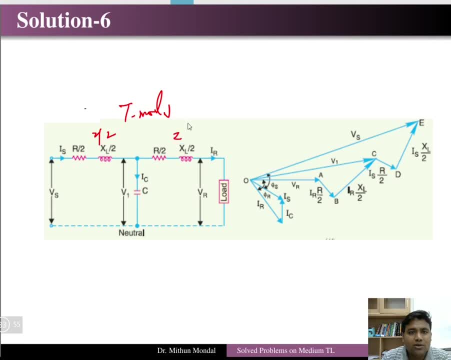 using. so this is equal to Z by 2. this is equal to Z by 2 and this is your admittance Y and this is your load connected. this is the sending and voltage, this is the receiving and voltage and this is the phasor diagram. 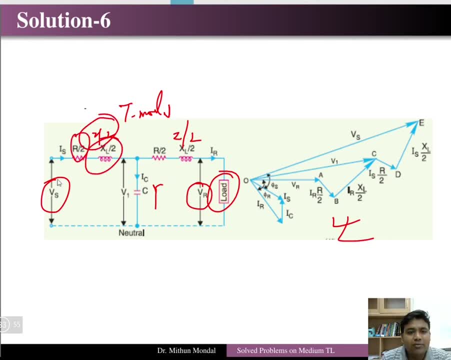 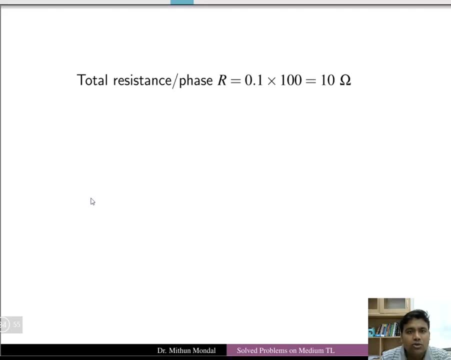 So here, since it is Z by 2, all the parameters will be R by 2 and XL by 2. here also, R by 2 and XL by 2 will be there. However, this will be equal to C. now, total resistance per phase then, since the length of the transmission. 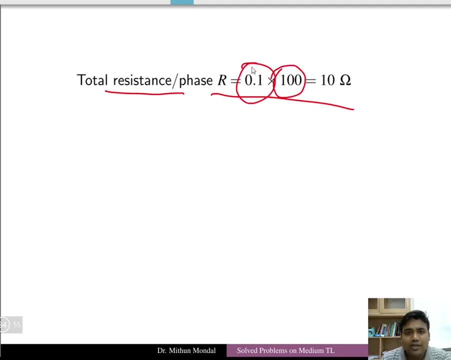 line is 100 kilometer and 0.1 is given. so multiplied so total resistance would be 10 ohms, total reactance multiplied with 100, 0.2, 20 ohms and capacitive, capacitive susceptance: we have to multiply. 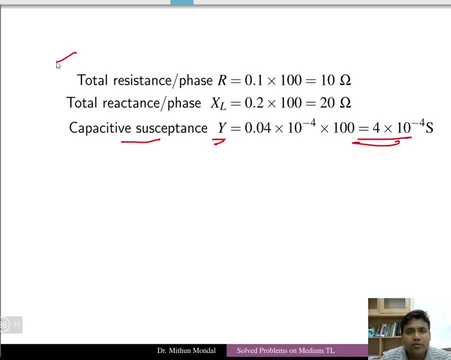 So it is equal to this much Siemens. so in this way we have find out the values of R, XL and Y. now we can easily can construct the, we can construct the T model where this will be equal to Z by 2. this will be Z by 2 and this will be equal to Y. So Z by 2 means R plus JX divided by 2 parameter. 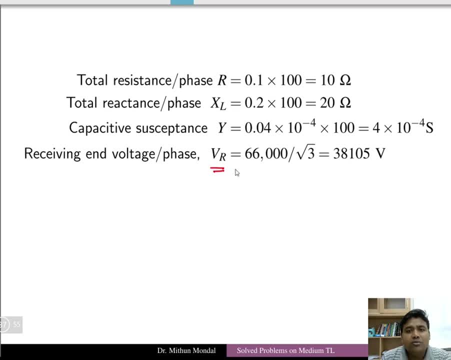 So the receiving and voltage would be equal to 66,000 divided by root 3, because we have to convert it in single phase quantity, so this will be 38105 volt. Then the current information. so this is the load we have. what is the current flowing here? IR. 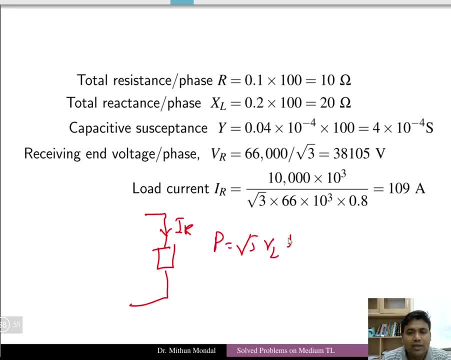 So we know that power is equal to root 3, VL, IL, cos, phi. So using this formula we can find the current IR. So power is given to be 10,000 kilowatt and 66 kV is given the voltage, so it is equal to 109 ampere. 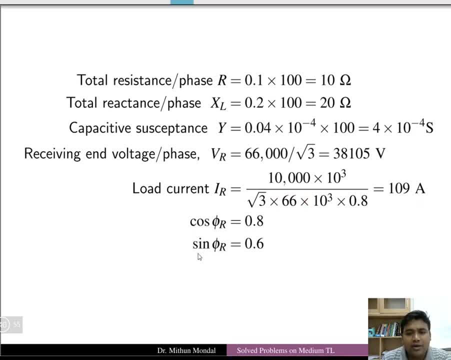 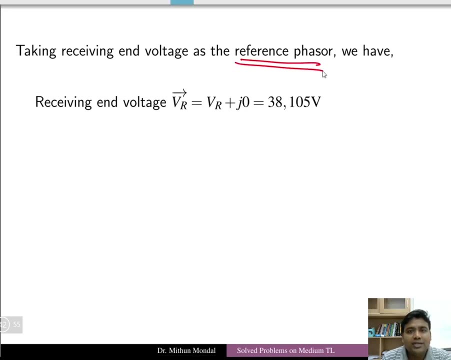 Cos phi are given to be point 8, sin phi R will get .6.. So the impedance of the line per phase is equal to Z, is equal to 10 plus. so 10 is the resistance and 20 is the reactance. And then the receiving and voltage will be taken as the reference phasor. so VR, this angle, will be equal to zero. 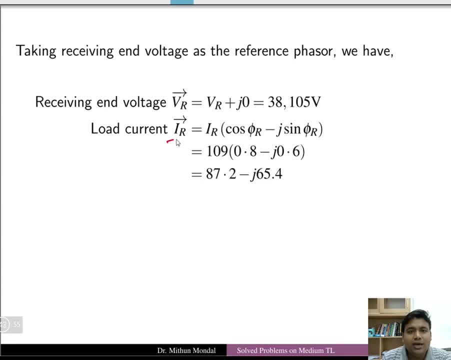 Then the receiving and current. you can take cos phi R minus sin phi R, So this is the receiving and current. We have to10000 dt find out the magnitude of the current and the engine. so the voltage across c, what is the voltage across c? so we can apply the kvl equation. so we can apply the kvl equation in this loop, so this: 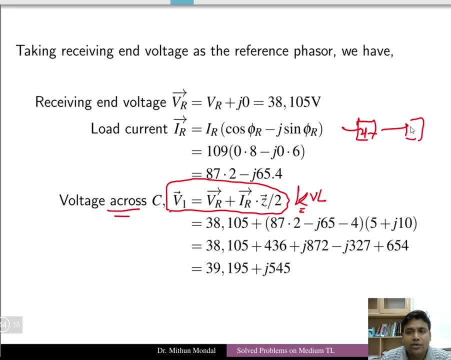 is equal to z by 2. this is equal to z by 2, and here you have the y right. so what is the voltage across v1? you have to find out. so this will be equal to the receiving and voltage vr plus the drop here, voltage drop. so apply the kvl in this loop. apply the kvl in this loop to find out what. 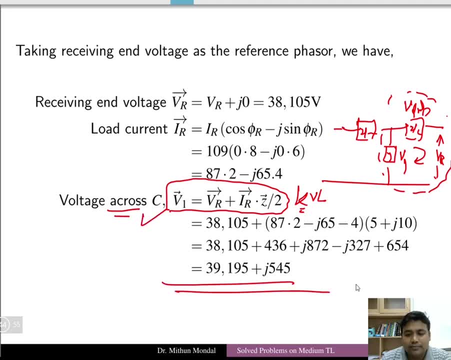 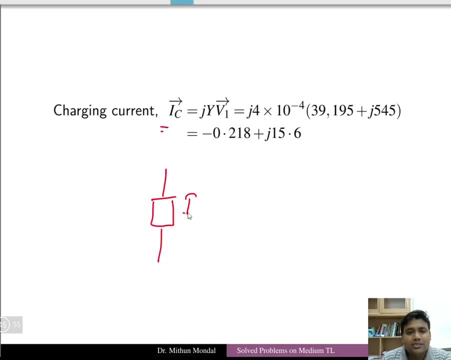 is the voltage across the capacitor, so you get this much. then the charging current, i see, because this is the sun parameter you have, so current is equal to voltage into admittance, where admittance is equal to j, omega, c, so that you can do to find out the charging current of the line. so the sending 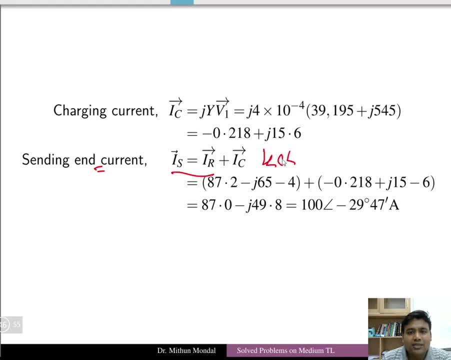 and current is equal to. so this is the kcl equation that you can apply, because the current is dividing into two parts. current is dividing into two parts, so this is the current ic and this is the current ir. so what is the sending and current is? so at this junction, you can apply the 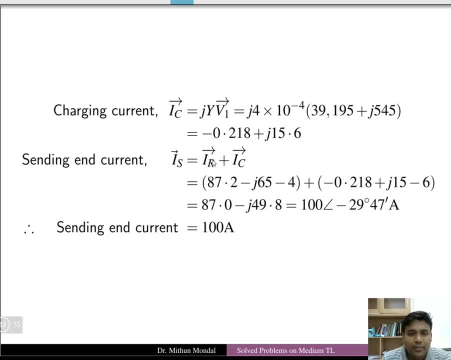 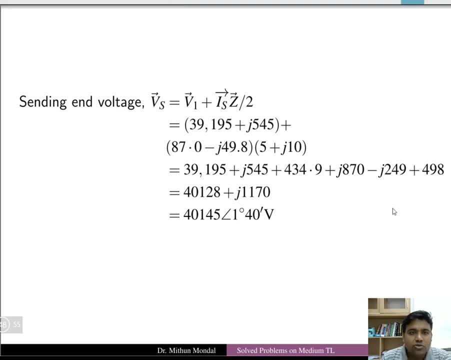 kcl. so is is equal to ir plus ic. so the sending and current magnitude is coming to be higher: 100 ampere, with some angle minus 29.47. so sending and voltage, now you can find out. apply the kvl in the first loop, so you can apply the kvl here. so this is equal sending and voltage. this is your. 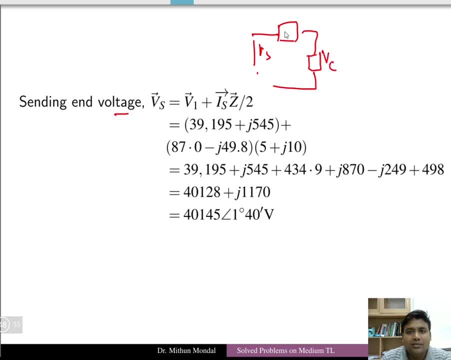 voltage across the capacitor v1 or vc, and this is the drop z by 2. so apply the kvl here. so once apply the kvl you will get this much sending and voltage. so once the sending and voltage is applied, so this voltage is corresponding to single phase. multiply with root 3 to convert it into line. 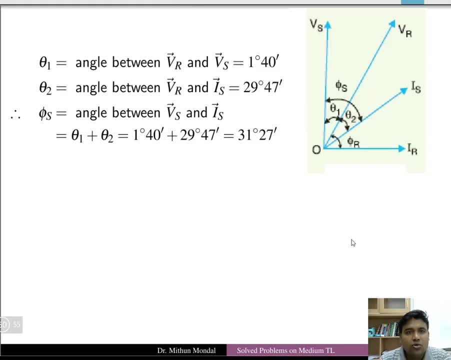 voltage of the three-phase quantity. so after that you have to obtain the value of theta 1 and theta 2. so what is the theta 1? theta 1 is the angle between vr and vs, so the angle between the receiving and voltage, and the angle between sending and voltage, the angle between receiving. 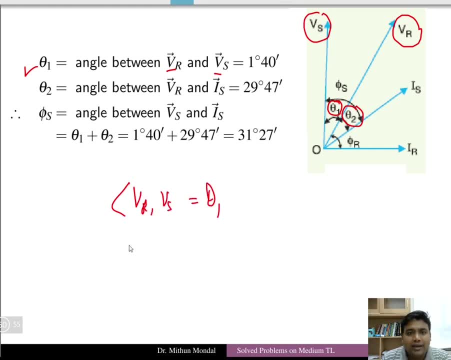 and voltage is the angle between receiving and voltage. so this is the angle between receiving and and sending, and you will get theta 1, and the angle between receiving and and sending and current. you will get theta 2, so the value of phi s. that is the sending and power angle between.